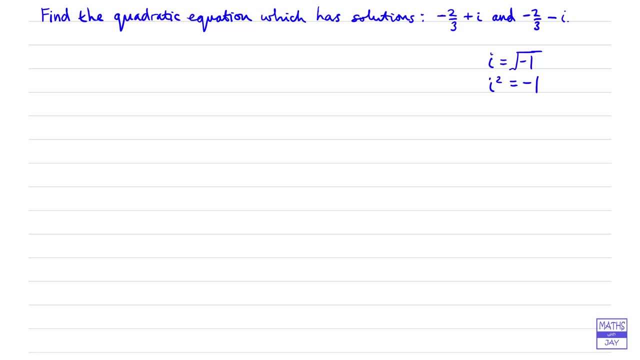 course that means that when we square it we get minus one. So i squared is minus one, And the other thing that's important is to know what we're aiming to do. So we're trying to write down a quadratic equation. So we know we're looking at complex. 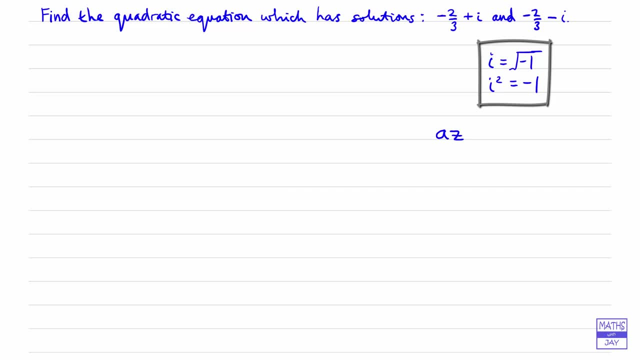 numbers. so let's start by thinking of the answer as z. so we're thinking of a quadratic equation that's going to look like a z squared plus b, z plus c is equal to zero. Now we can see that the solutions that we've got are complex conjugates, in other words, the 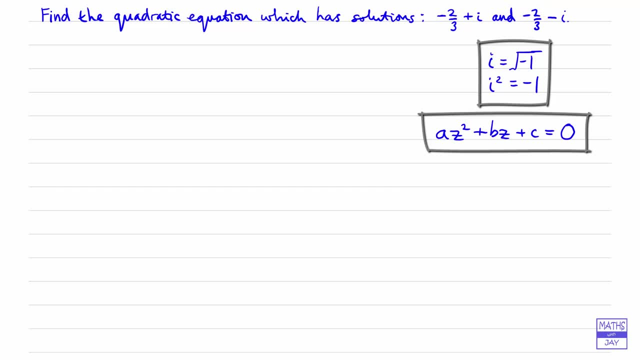 the real parts are the same and the coefficient of the i is plus 1 in in one of the roots and minus 1 in the other. so we know that a, b and c are going to be real numbers. So we're looking to find the quadratic equation: a, z squared plus. 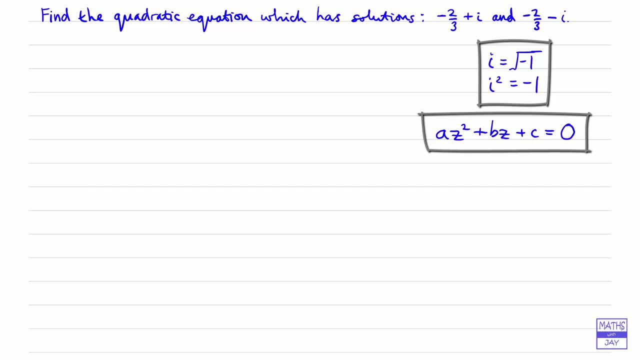 b, z plus c is 0, so we know where we're headed. So now let's go back and think about these actual roots and think what we're going to do with them. All we need to do is say: well, we know that we've got z minus each root, so we start with the. 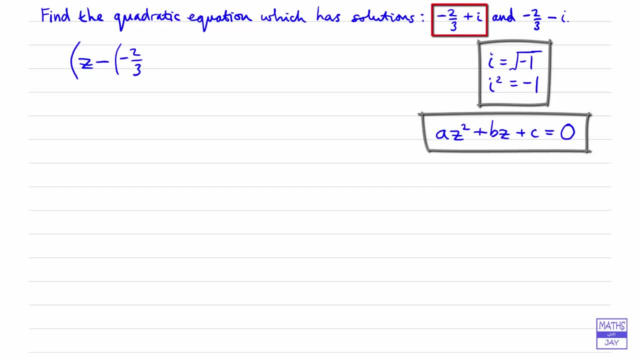 first one. so minus negative two-thirds plus i, multiplied by, and then we put the other root in here, so that's going to be minus two-thirds minus i. so we know that the product of those two things is equal to 0, and all we've got to do is multiply. 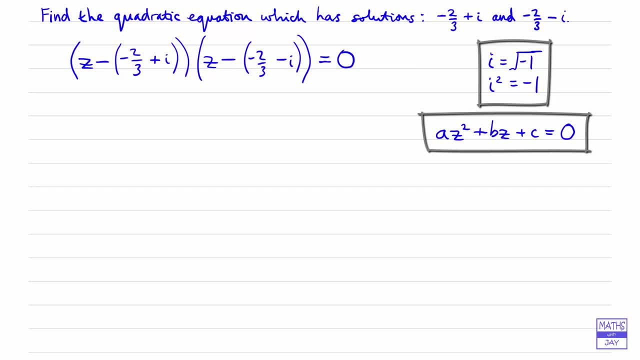 that out and simplify it until we end up with a z squared plus b. z plus c is 0, and then we're done. So let's first of all get rid of the brackets inside the brackets. So here we're going to have z plus two-thirds minus i, and in the second bracket 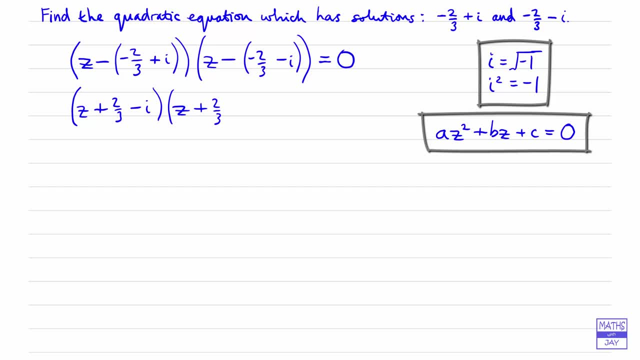 starts off the same plus two-thirds, but this time minus minus. i will give us plus i. We can see that the first part of the bracket, the z plus two-thirds, appears in both of them, doesn't it? So I've highlighted that, because then we can see. 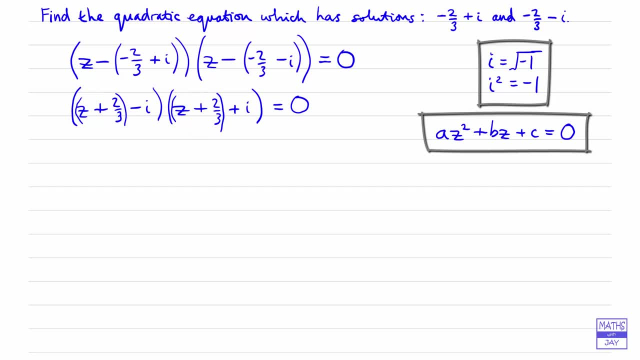 what we can use next is the, the idea of the difference of two squares. So, for example, we know that if we're multiplying x minus y by x plus y, that's the same as x squared minus y. So that's really what we've got here, isn't it? We've got x is z plus two-thirds. 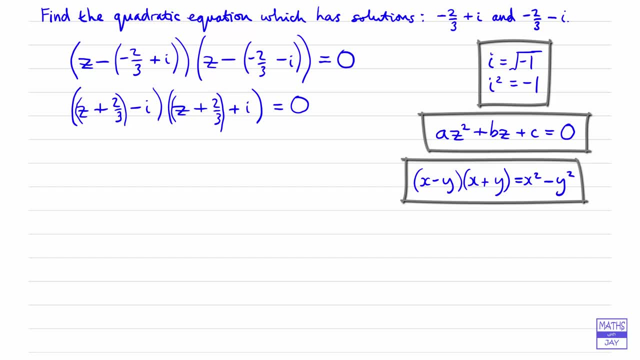 and y is i. So that means that when we multiply this out, all we need to do next is write z plus two-thirds squared minus. i squared is 0.. So then, multiplying out the bracket, we've got z squared two, lots of two-thirds of z. so plus four-thirds z and 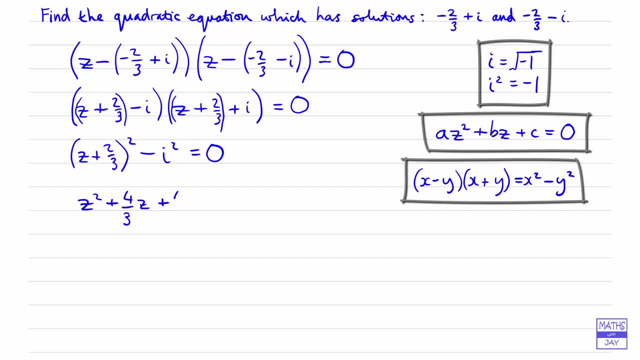 then two-thirds all squared, so that's plus four-ninths. and then, remember, we know that i squared is negative one, so we're subtracting negative one, in other words adding on one, So we can take together the last two terms, so the z squared and 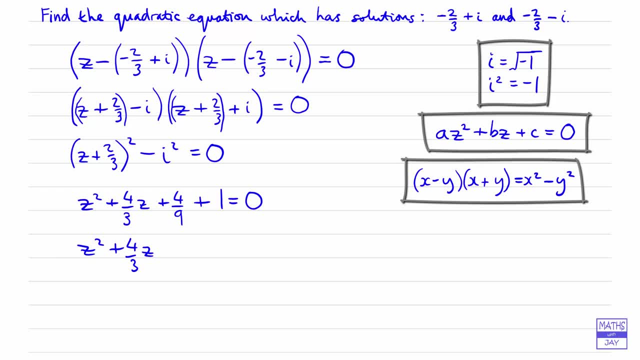 the four-thirds of z aren't going to change at the moment. and one plus four-ninths, well, that will be. well, one is nine-ninths, so that will be thirteen-ninths, and then, although we could say, well, yes, that's a quadratic, I think it would be. 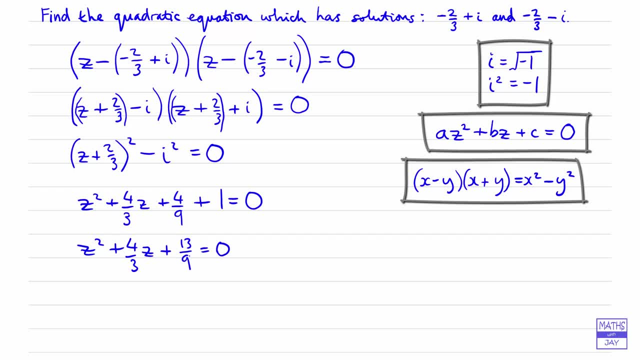 nicer if we had whole numbers multiplying each of the terms. so let's multiply through by nine, So that will give us nine z squared plus, and then nine divided by three. Three times four is twelve, so we've got twelve z in there, and then nine times thirteen-ninths will be thirteen, and that's equal to zero. So we've done what we were asked to do. 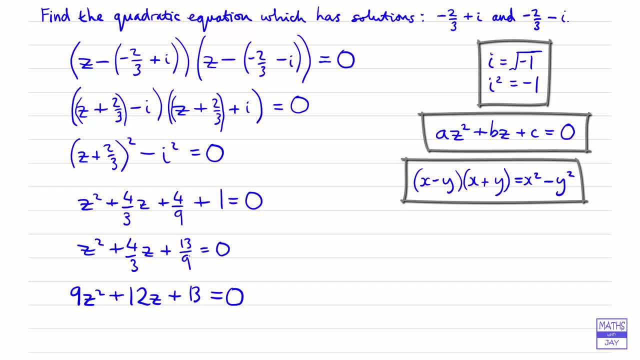 found the quadratic equation, which has the given solutions. If you want to check that, you could substitute in either one of the solutions or both of them, or you could start with this equation and solve it either using the quadratic formula or you could complete the square. or if you had a calculator that would solve this sort of equation, you could try that too.